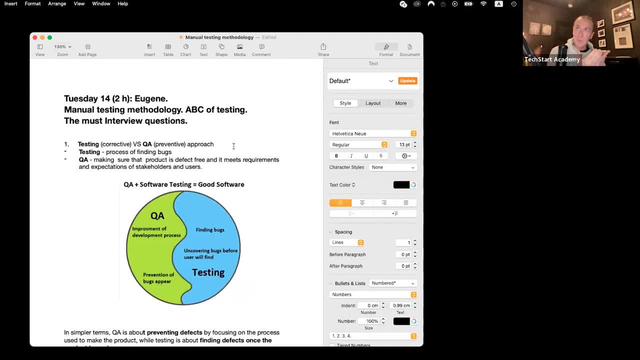 created it. It's here on my computer But I'm reading documentation. It's like hey user is supposed to be able to log in and send the message to a medical provider, whatever, And I'm testing it Like before it's been released. When tester starts working on this. 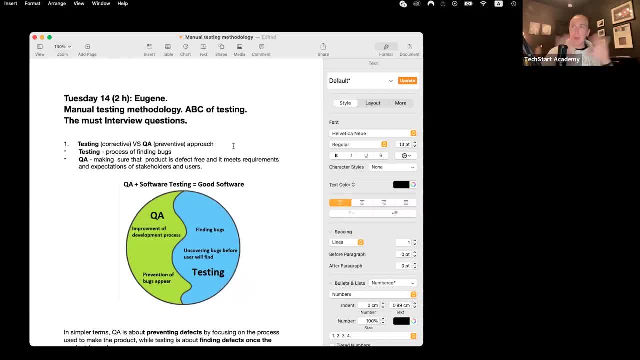 application Tester. So you might do this without any documentation Because, like hey, imagine that you are a user and do whatever user would do. So it's a very good interview question, Because sometimes people just can't separate these two terms: Quality assurance and testing. So in this, 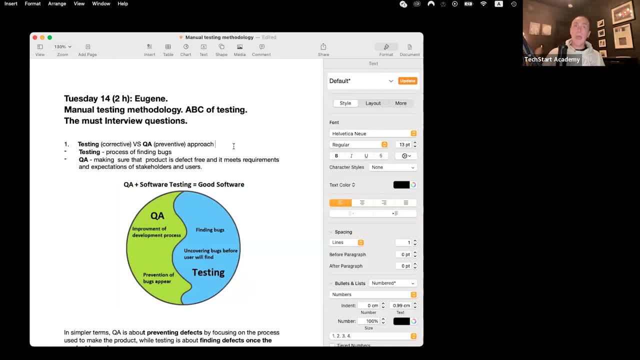 case: testing, this is corrective actions, And quality assurance, this is preventive approach. So we We are using these two terms. So this is corrective, This is preventive approach, And Quality assurance: engineer starts earlier. Tester starts doing his testing after product is created. 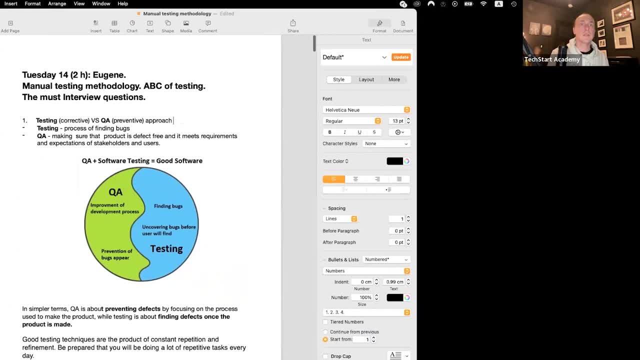 So this is very important thing And here's the picture about it. So, yeah, quality assurance, this improvement of development process and prevention of bugs to appear. They will appear anywhere, but you try to prevent And tester finding bugs and uncovering bugs before user will find it. 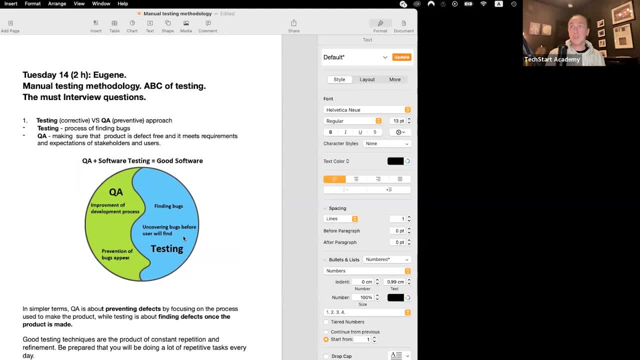 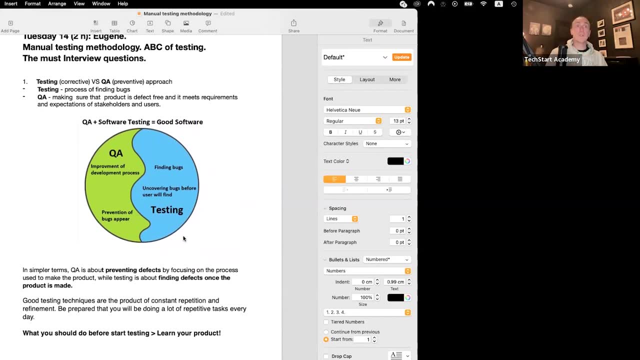 Because first application goes to testers and then goes to users. Okay And yeah, I will share this lecture with you as well. And, in simple terms, QA is about preventing defects and testing about finding defects when product is made. What you should do. 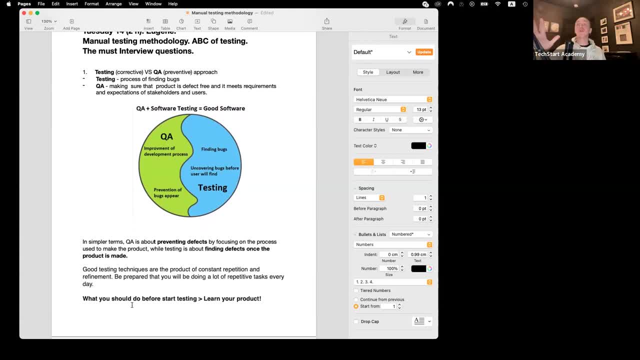 Before you start testing, no matter who you are, quality assurance engineer or you're a tester- Actually there is no position like I'm a tester. Usually we do both. It depends on the situation. But anyway, no matter what you do, 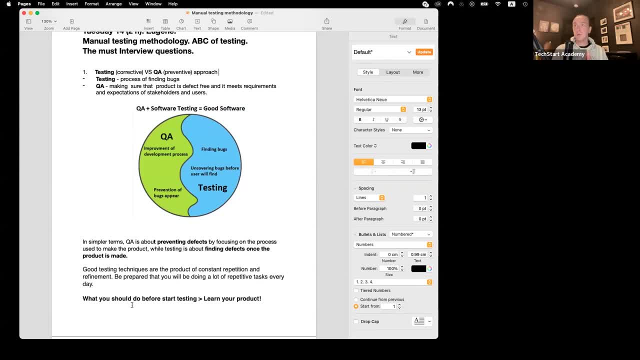 And before you start testing, you need to learn your product, Just as a customer. for example, There is New social media, I don't know Kind of Instagram. What you would do. You install it on your device. What is the main purpose of Instagram? 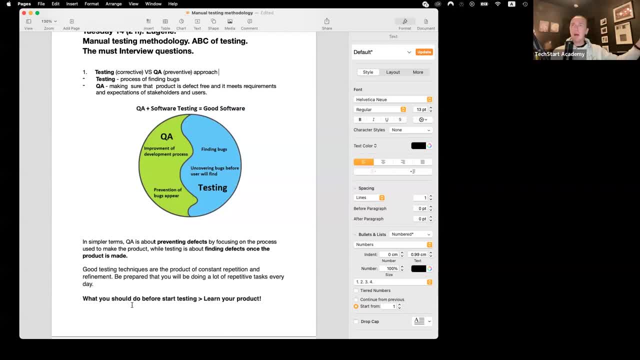 Make a picture and share it. Nobody cares about this. menus Like how many features it has. First thing: Yes, of course you, you should be able to log in. This is like. it means your application is in testable condition. 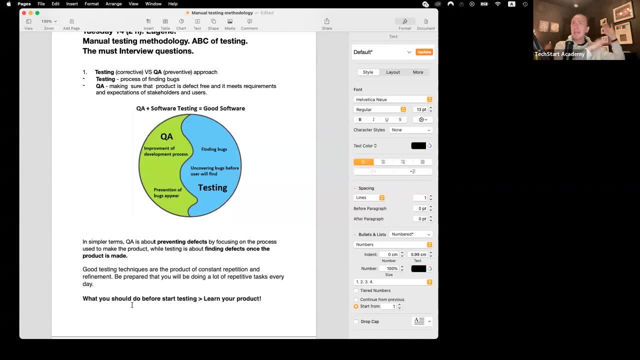 If you can't log in, forget about any. everything about menus, about pictures, about Everything. I just can't log in, So this application can be sent to the apple store, to the play store, anywhere. Yes, It's all about making picture. 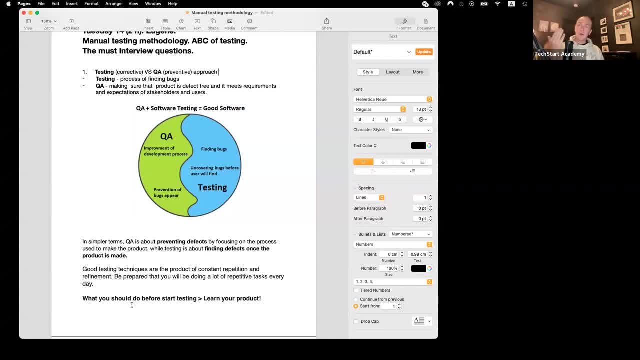 I want to make a picture and share it. It's called happy path. You, as a user, can log in, You can make a picture, share it. You're done. This is your happy path. If you can't do this, you should. 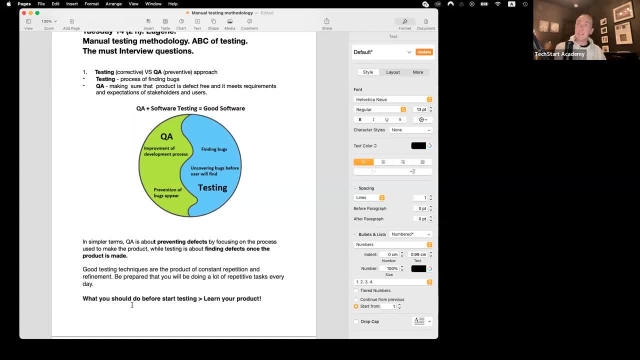 Stop testing. You should create a meeting like guys. It just doesn't work as expected by testing Just one feature, because it's all about this. I don't care about any other features. I want to share my picture, So the- and this is how we start learning after this. 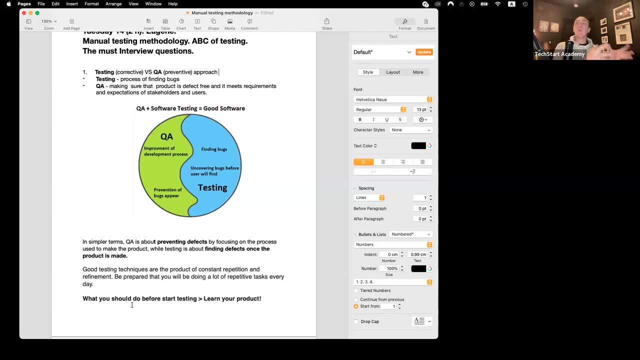 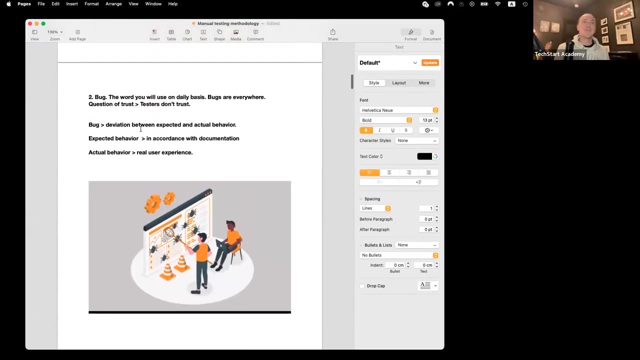 If we were able to make our happy path through application by logging in and sharing the picture, then we can learn about this project. Select all the possible features, whatever we want. Like, Hey, what this application can do. So here is the bug. 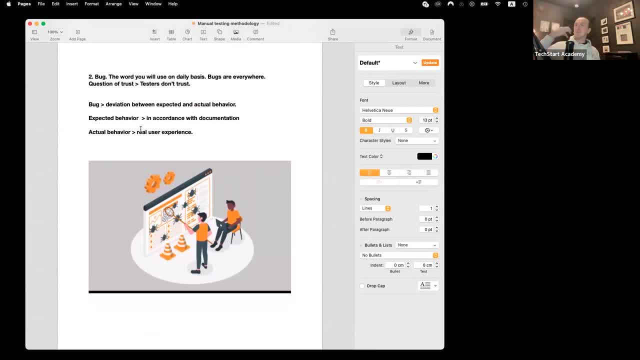 Yeah, this is the word you will use, You will say, you will hear on daily basis as a quality assurance engineer, because bugs are everywhere, literally every where you is just a question of time to find them. So, So bug. this is deviation between expected and actual behavior. 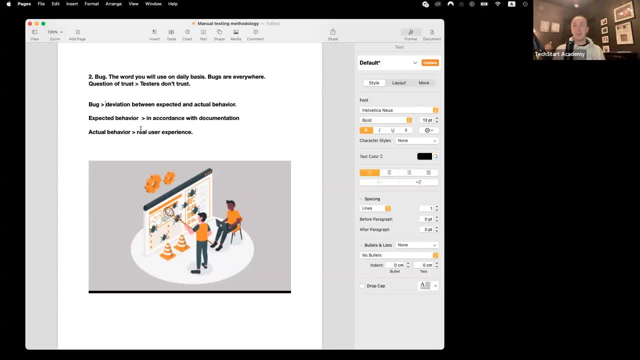 As a user. I want to log in to this application, to Instagram, but I can't. Here's the bug. I expect to log into this application but I can't for some reasons: for code problems, data problems, network problems. 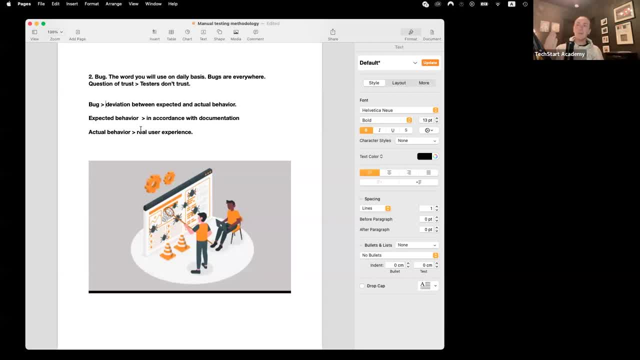 I don't care, I just can't log in. This is the bug. but since you're a quality assurance engineer, you should care. You should care why you can't create a ticket just by saying like I can't log in. 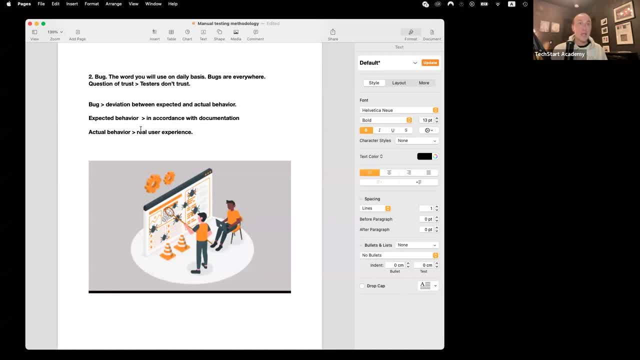 You need to provide some information, but we will talk about it later. So, yes, a bug. This is deviation between expected and actual behavior. expected behavior: This is the behavior in accordance with documentation, right? So I am as a developer beside like yes, user is supposed to. 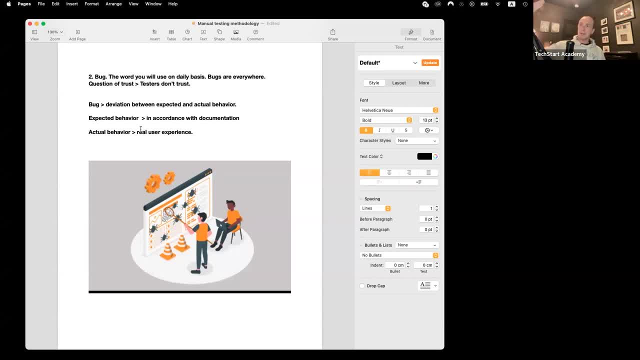 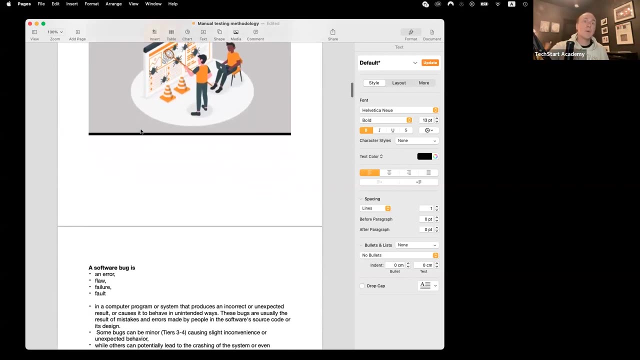 Log in If user provides a name and password, Okay, But actual behavior- this is really user experience. User has no idea what developer had in mind. Like he created account But can't log in. Okay, Why it happening? So yeah, this is like the full explanation of software bug. 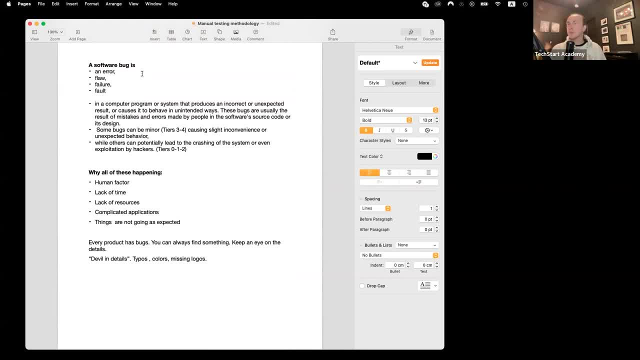 This is my like an error, failure, fault. Which word were uh? which Word, Which word works the best for you in computer program or system that produces an incorrect, like a blue screen, or unexpected result or causes it to behave in unintended ways? 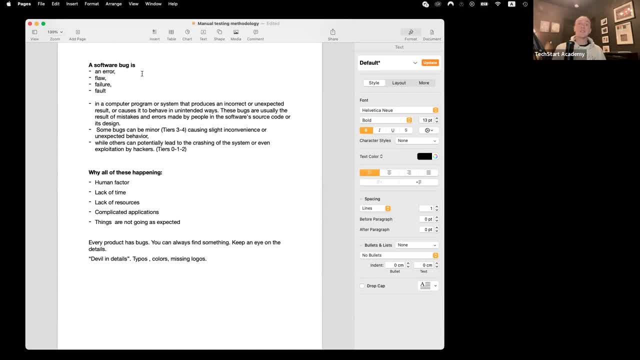 Uh, these bugs are usually results of mistakes and errors made by people in software source code: bingo or design, maybe button in the wrong place when someone knows uh, and some bugs can be minor. We will talk about triaging. 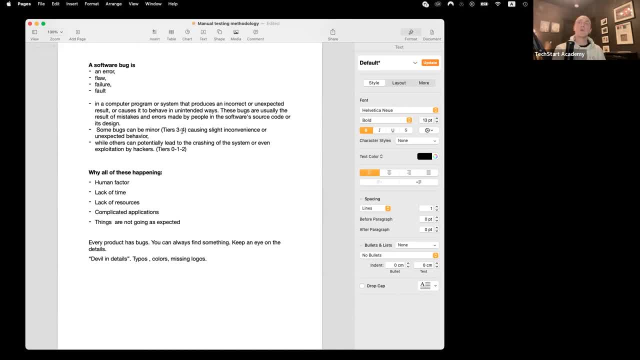 This is a new word for you, I believe it's tier three or four, like low priority, And we and tier zero one, two very serious, severe bugs which lead to crash of the system or exploitation by hackers. Why do you think bugs happening? 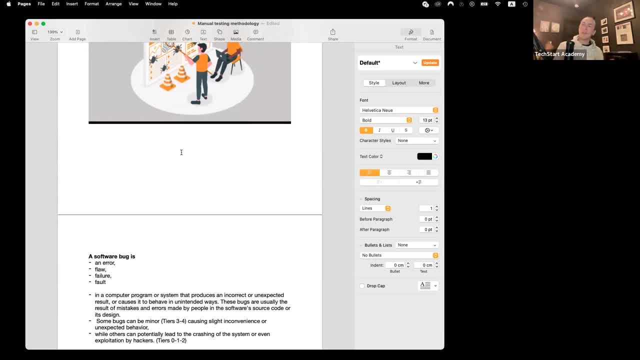 Why developers, when they write code, they do their best, right They they get very good salary. They are very dedicated people. but why bugs happen happening? Why? why we? we still can't find them human factor? We're all humans. 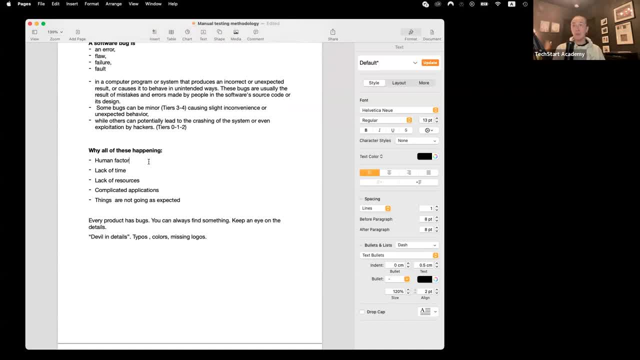 People do mistakes And, uh, sometimes other people. when they're checking someone else's mistake, they skip them because we're all humans. Okay, Lack of time, because we never have like enough time, because it's everything like: Hey, Hey, let's do it. 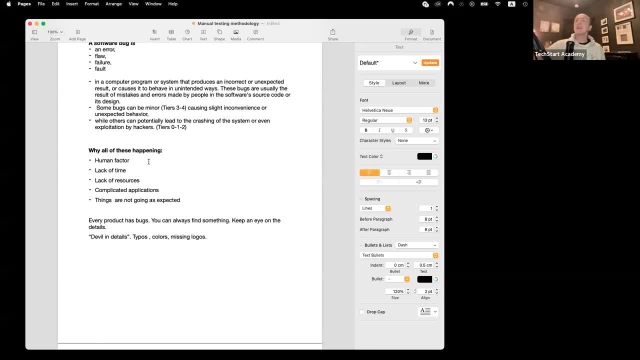 Let's do it because we need to build this application, go to the market, get our million of people money and so on. Yes, Lack of resources: We don't have like. I would like to have like 10 developers, but I have budget just. 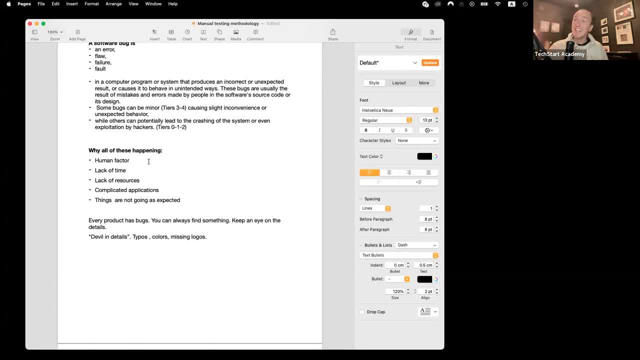 for three and and one or one, and these developers might be in different places on the planet. and, yes, sometimes one developer Created some like create a feature or hotfix in production. just pulled it there immediately And another guy on the team had no idea that it happened and it's like, Oh my God, you. 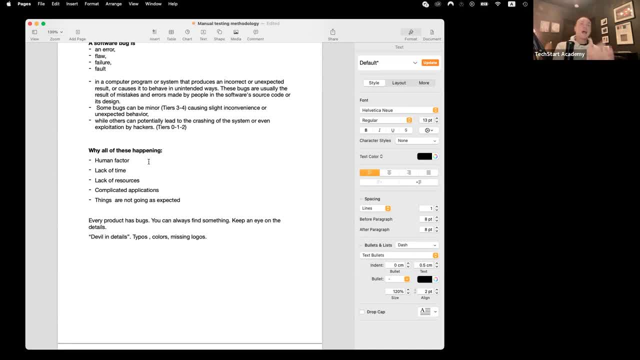 should have told me it happens. It happens, Anyway. complicated application: Yes, All these applications these days are very, very complicated, Especially if you work with media like Instagram, TikTok, because people have a lot of- um, uh, some of the most everybody's silicones. 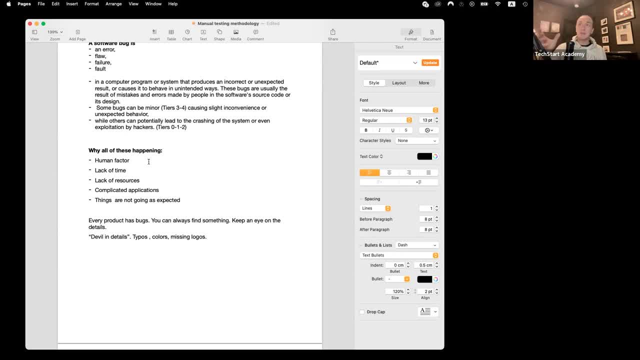 Okay, People, uh devices this day, all these devices, different version, different versions of um software, different versions of uh application, uh, they're trying to upload these different files, video, audio. that's just crazy, but it's. it's about fun. it's about having fun, but for me- i work in health. 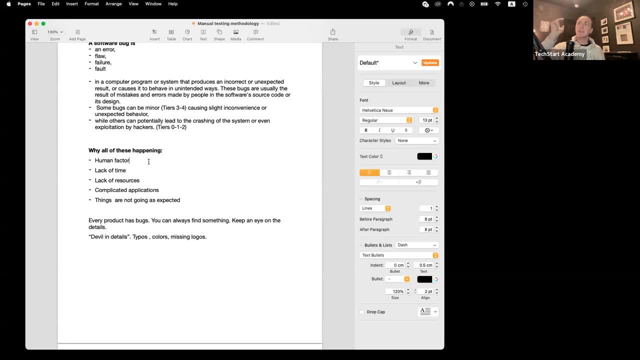 industry. we have billing, we have uh this, uh hipa, uh protected documents, uh encrypted, non-encrypted, uh messaging is just insane. how many features? because we need to protect our customers. or imagine that you work like in a bank application. it's just crazy. testing billing, it's, it's. it's a different level, seriously, and it's so complicated. so, yes, 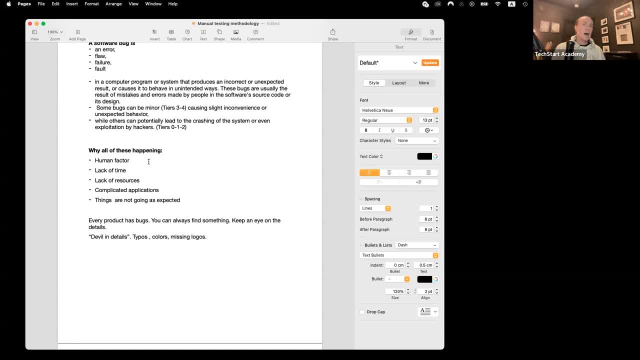 this is another reason, because you can't, uh, imagine all the possible use cases, i mean, what real user can do with this application. sometimes people do crazy things and applications and they're expecting this application to work. so, yes, and the last thing, yes, like things are not. 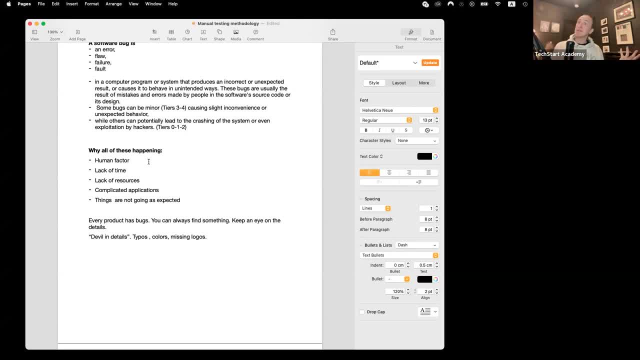 going as expected. like, like you know, it happens uh and yes, uh, my um idea that is: every product has bugs, every, i swear. i mean, if you try to find bugs on facebook or google, of course it's so hard to find them there, but if you take a look at very basic 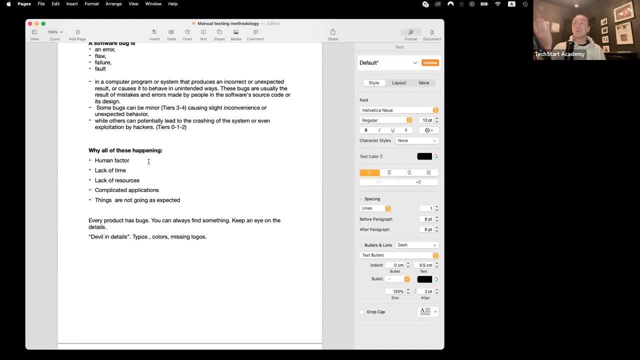 applications like i don't know. maybe your insurance company has an application and it's not huge. go and test their application. you find a lot of bugs because they, like, they don't have budgets. they have maybe a couple of developers there and these poor people they are trying to. 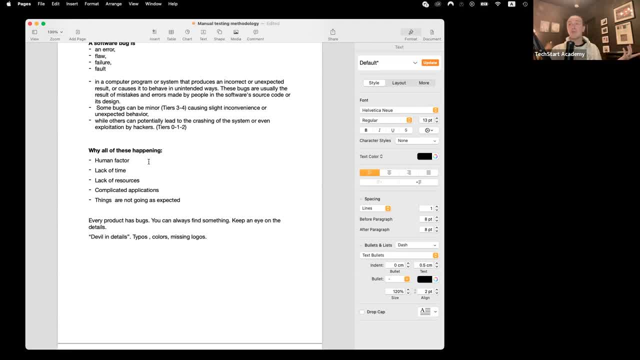 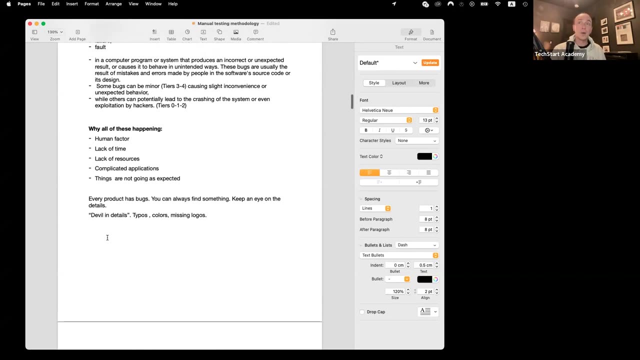 create. or, for example, my daughter goes to a school and we have school application. seriously, they saved some money on quality assurance, that's for sure. but just um, yeah, i will show you some examples, uh later. but yes, uh in. and all this like top applications, like instagram, as i said, it's hard. 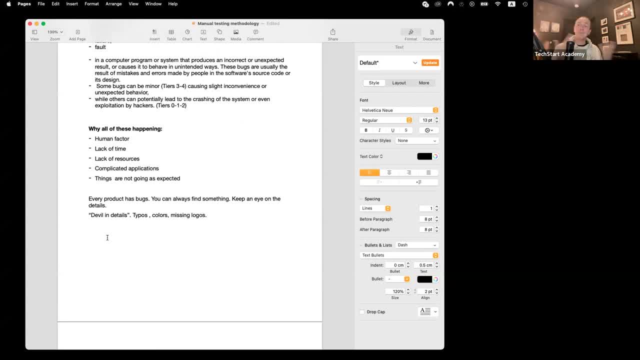 to find any bugs, of course, but for the like, very basic stuff, for the like stores, application insurance companies, some small clinics, if you start testing them properly, i mean just manually- you will find like one bug per hour, i i promise you. and yeah, i noticed the uh, this part, that's. 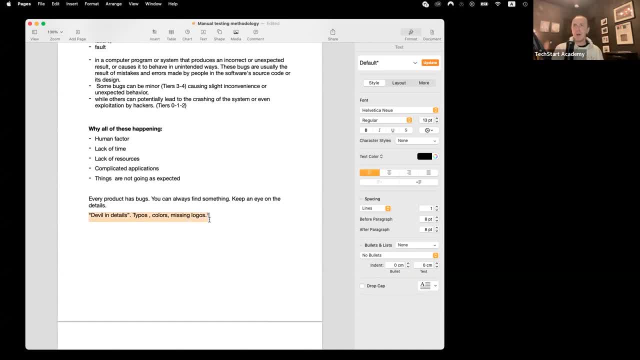 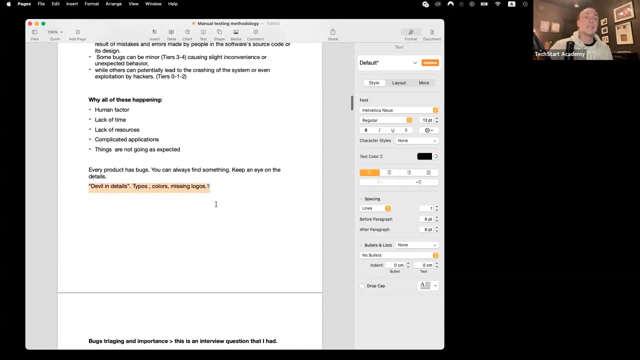 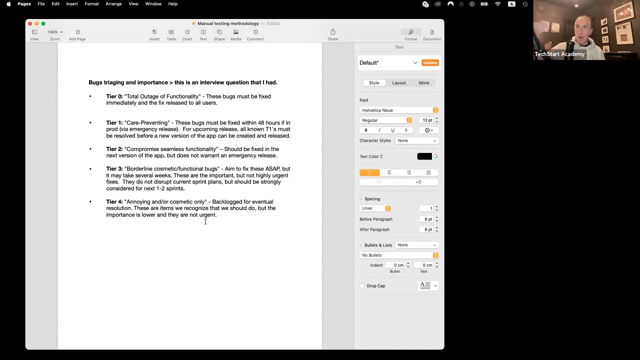 like devil in details. uh, don't expect that application will be crashing or you can't log in. no, just take a look at the details, like colors, uh, calendars, date selectors, all that stuff. there are a lot of mess there, usually there. uh, so next bug tragedy? this is basically how we rate our bugs: from zero to four. it's from my company. 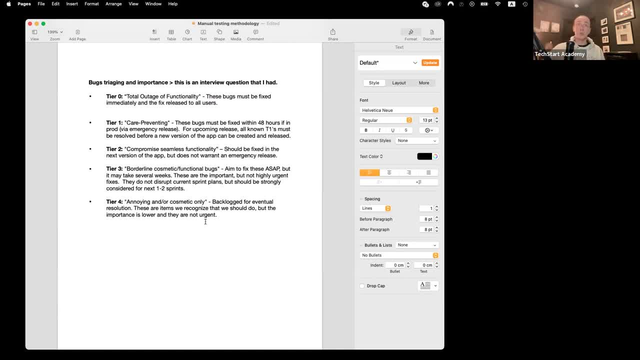 i mean, maybe in other companies that might be from zero to three or from one to four, but uh, when you create the bug, you need to understand its severity, how it affects all the system and if you can't log in or application crashing, this is tier, tier parousia. 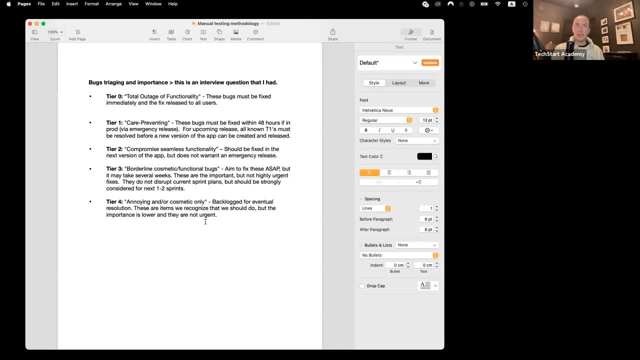 so tier zero is total outage of functionality. it means it affects all the users and we should fix it immediately. right now, users can't log in, application crashing uh. you can't buy, uh a product on amazon, so it means like potty is over, so we need to fix it. uh to your one. this is very. 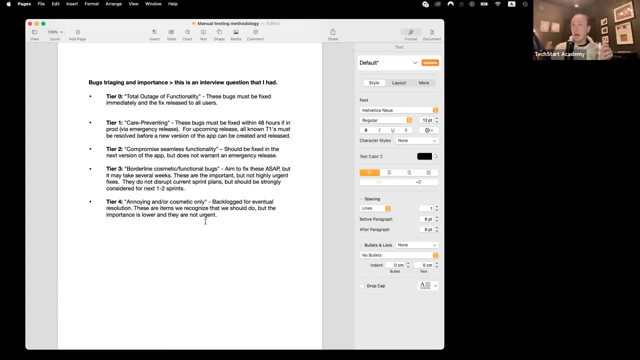 important bug and it should be fixed within 48 hours. uh, so, for example, user can use the application, but something important just doesn't work. usually, uh, uh, you will not be making decisions about this triaging. Usually, your product owner or team lead will be responsible for this. 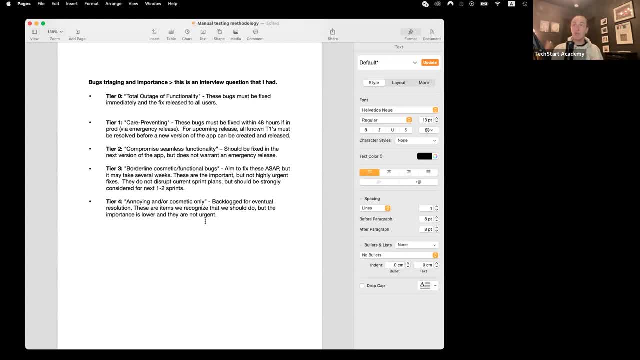 usually, but you need to know what does it mean? So if we have like a tier zero, it means everybody is dropping what they were doing and fixing this bug. Tier one: we have like 48 hours to fix it. It's something very important. Tier two: this is like compromised seamless functionality. It's like 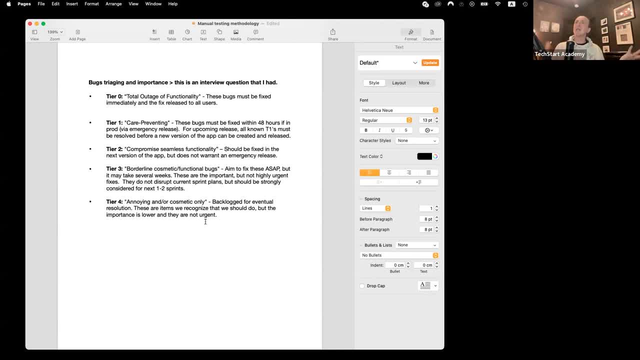 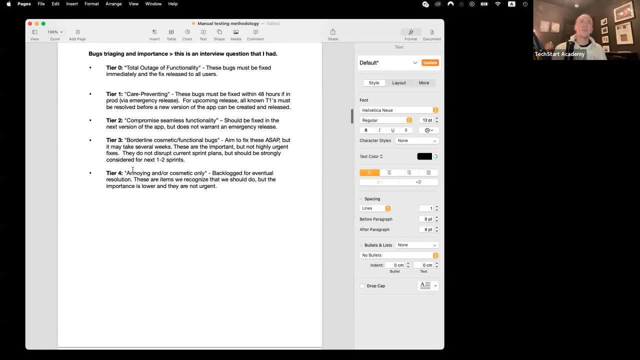 I mean something is not working, but it's fine, because not so many users use this feature. or I mean, and three and four, usually they go together- Tiny bugs it's. usually they never be fixed. Your application is supposed to be tested all the time, But when we're talking, 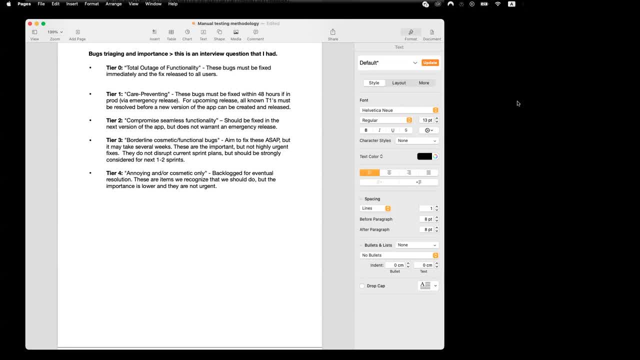 about production. this is the environment for users, for customers. It's supposed to be tested as well, And usually for this we just run automation scripts and making sure that everything is working. But I mean, technically it's just impossible to test it like every hour, every day, like because we need to test other features. 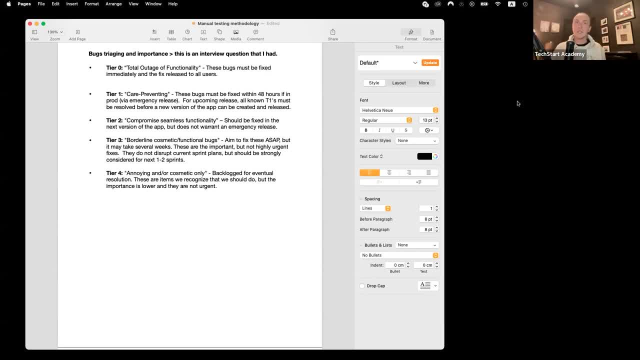 We develop our application, We're adding some new stuff. We have three different environments: UAT, user acceptance, development or staging, and prod. And imagine how many people do we need to test all the features in all these environments on different devices, especially if we're talking. 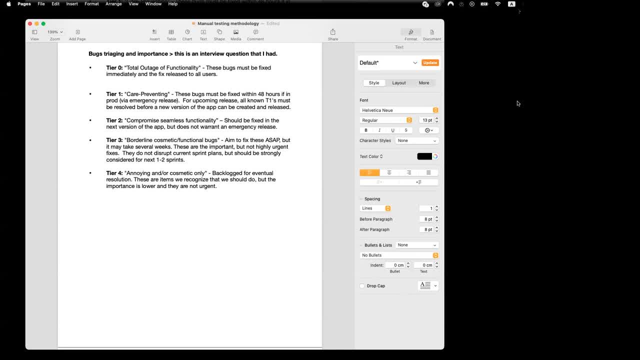 about devices, at least on iOS and Android, on Windows and Mac. That's insane. That's why we were talking about earlier lack of resources, lack of time, lack of people. We just don't have people and time to test everything And that's why it's happening. And when you get complaints, 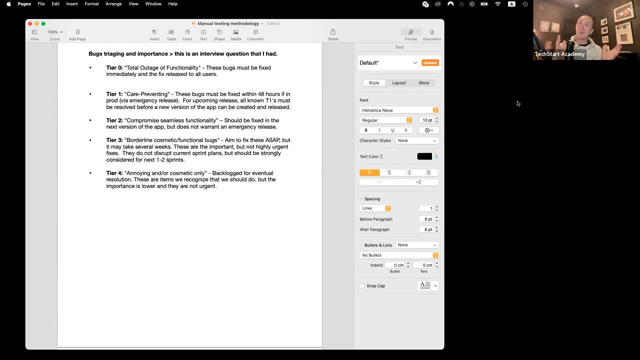 from the users. that's catastrophic. You're supposed to get complaints from testers. Users should not have any problems. Anyway, as a tester, you will be testing, That's easy. But I mean what you will be testing: UAT or production, Because customers don't work in UAT. 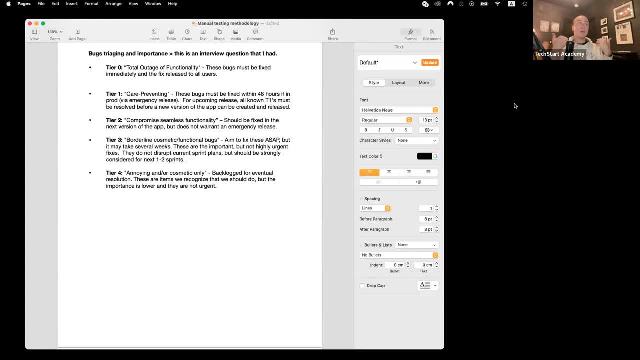 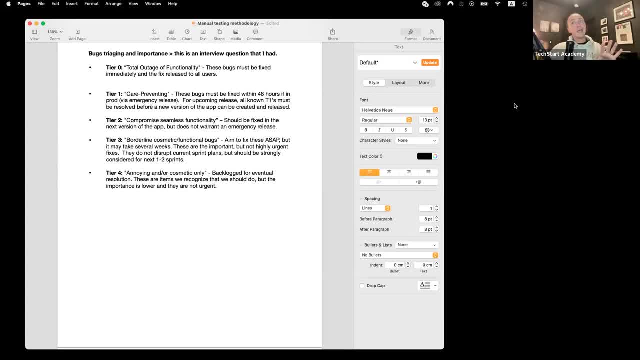 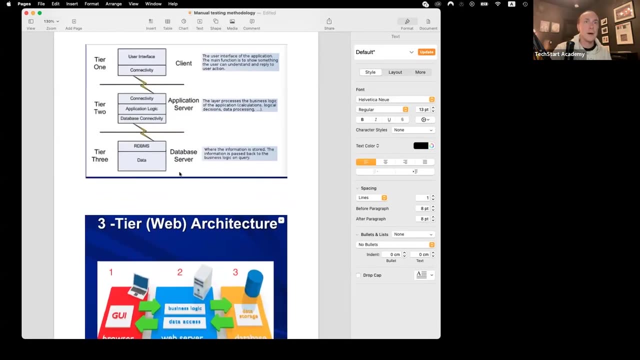 we care about UAT and staging, We just rely on environment, on production environment, like hey, it will work. So yeah, but this is reality And yeah, this is. you can take a look at these pictures when I where I'm trying to explain this trashing. 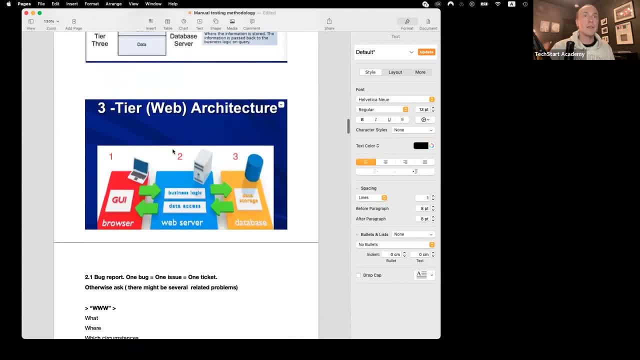 But this picture is more complicated, But this one is easier. So tier one, they're, they're all here. I mean, this is your computer, This is graphic user interface, This is your browser, So user here. So when tier one bugs, therefore users bugs, customer bugs. Tier two, it's something. 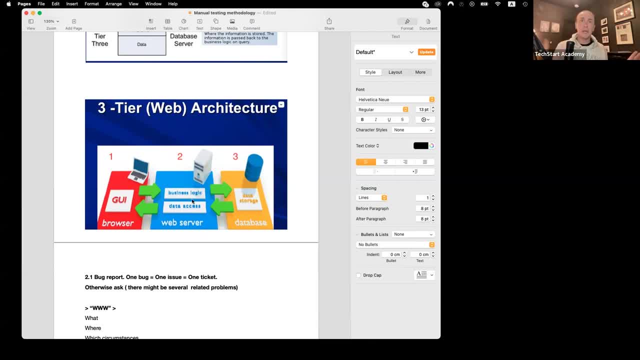 wrong with the business logic. A customer has no idea about it, But you as a tester should know like something is going on. you know we just added some data And user can see it in UI and something like this And tier three. there is something very deep in data storage And possibly 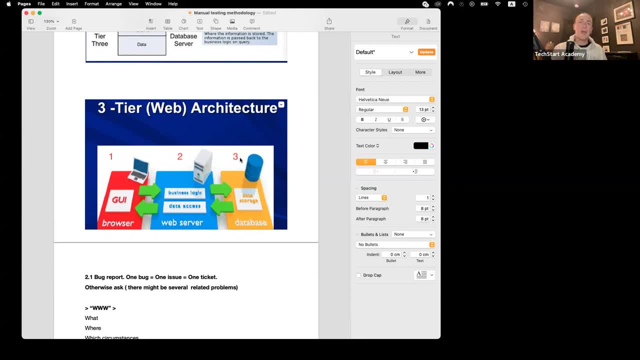 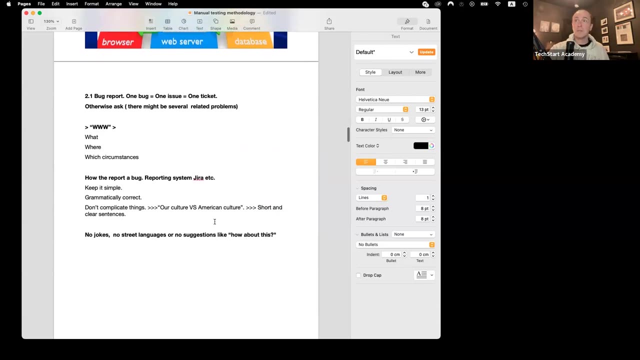 this is going to be like a developer's problem. They didn't update their database or they were playing around with resources, So it's really like developer stuff, But it's still going to be really important. Okay, Bug report. So we found a problem, Now we need to report it right. So 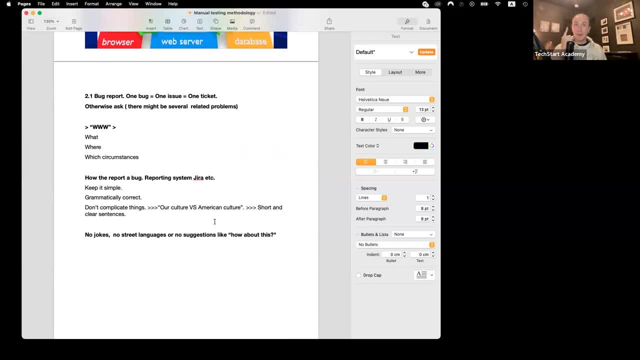 first rule: One problem, one ticket. We create one ticket, one bug report, which is the same for one problem. Just remember this rule. Like, we have this problem: User can't upload picture in Instagram. User can't create product in custom builder project. Here's going to be one ticket. You can't. 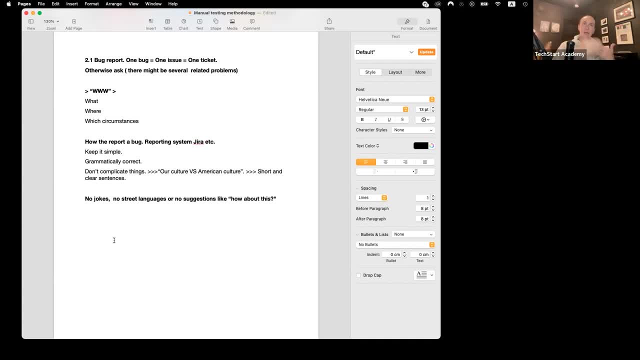 log in One ticket. Sometimes there might be like related problems And your team lead can tell you like hey, these three problems are supposed to be in the same ticket. But it happens rarely. It happens, but usually just remember: one problem, one ticket. 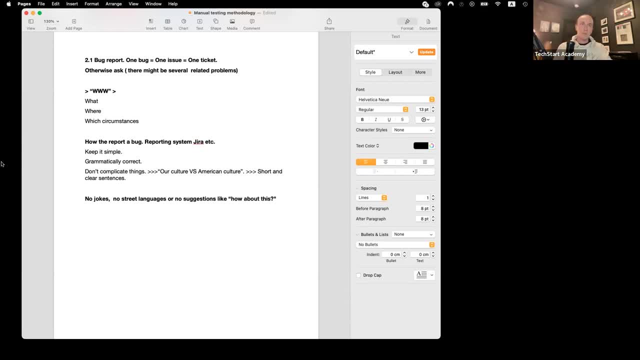 Okay, Talking about bug, What is the bug? Just remember these three letters W. So it means what, where and which circumstances. This is description of a bug: What happens, where it happens and under which circumstances. For example, I what you guys were talking. 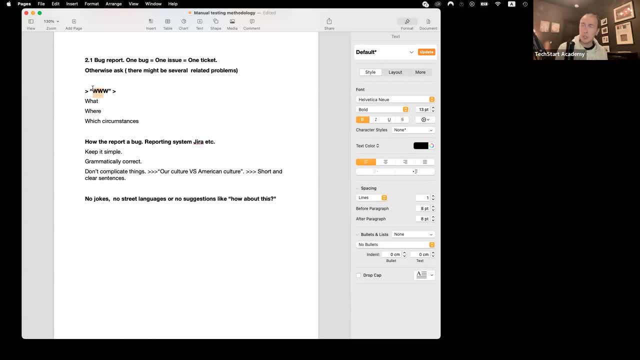 about this store that you couldn't log in. Here are like three things. I can't log in where on my laptop operation system, blah, blah, blah on in on Shopify application which circumstances invalid password. This is the bug report, So an overall keep it simple. 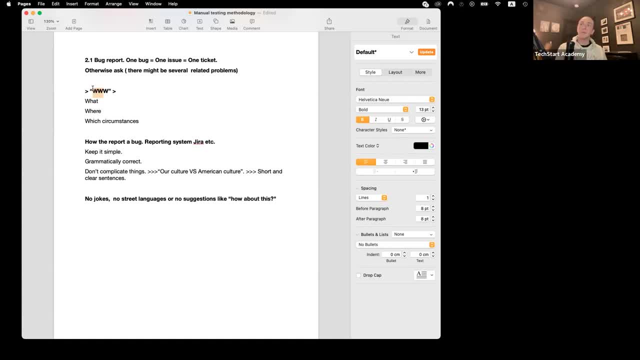 because people- I mean developers- who will- will be going through your description. they don't have time, they don't want to read all this blah blah blah, you know? so not so many details. just provide all the necessary details and we will talk about them later. grammatically correct: these days we have a lot of applications. 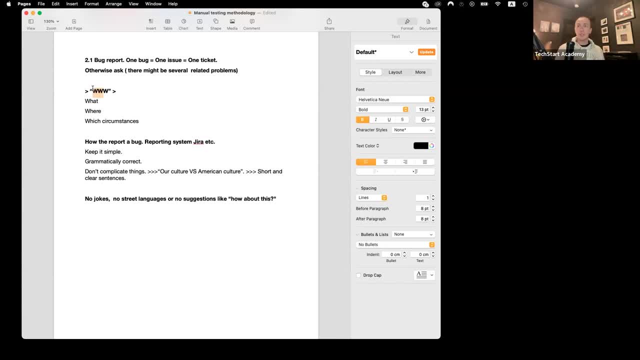 grammar, chat, gpt, whatever. just if you're not sure that you're clear, just take it, copy, paste it in your google translator in the grammar and just double check. everything is looks good. uh, and, as i said, don't complicate things, because i notice in american culture they really keep things simple. 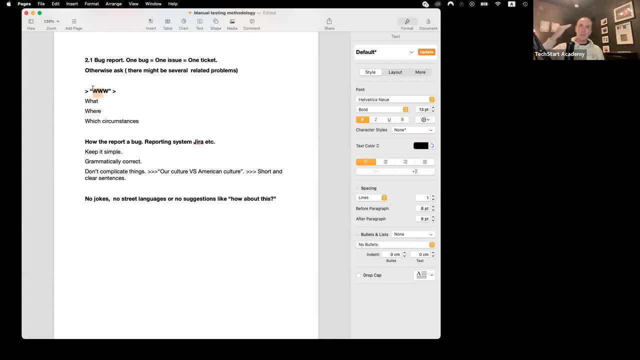 they use very short sentences. it's supposed to be like one, two, three, because they don't use a very complicated structures like we use in our languages, like oh my god, like for, like like this. no people with people who will read it. they just lost in there. just keep it clear and simple. no jokes, no like street. 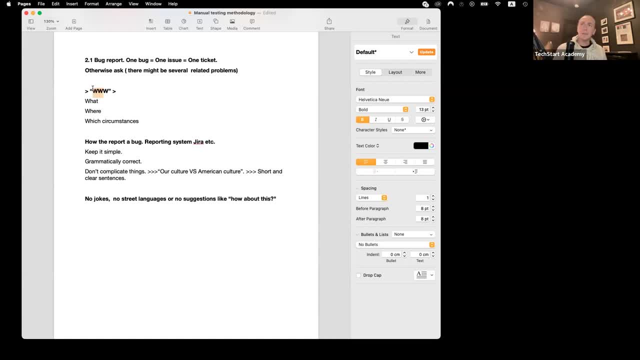 languages. no, no, like, just try to be professional. and so this is the example. like, uh, just for you, so like name, so name of the bug. user can't log in platform platform mac os, um, windows environment production. no, it's staging actually, whatever, it's not super important device browser. 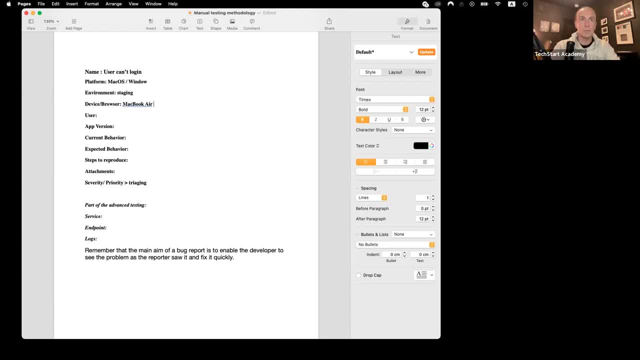 so macbook air 2 and um windows. so tablet, for example, user uh. if you have uh and uh, you have user novo, you can test: has less 8 Dead. my own uh uh, but this is basically uh, it's. they're. they're right now, then using uh, one more uh and it's the user'ming and they'll do stuff. 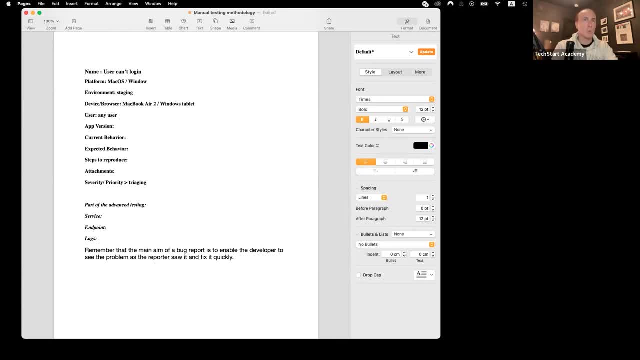 will hurt in the region of this application. um, and taking care that, um, so user user for this application. um, it was like any, you can say like any user, because nobody was able to uh, login right. app version. i don't know the app version for sure, but let be it like 1.0, it doesn't matter, you can take. 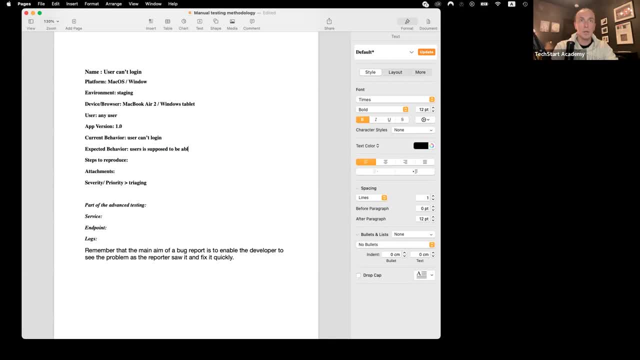 a look at the site. current behavior user: uh, can't log in. expected behavior user is supposed to be hey able to log in to their application steps to reproduce. here you can do like: open the app, provide username, provide password, observe, observe error message, and here you can. 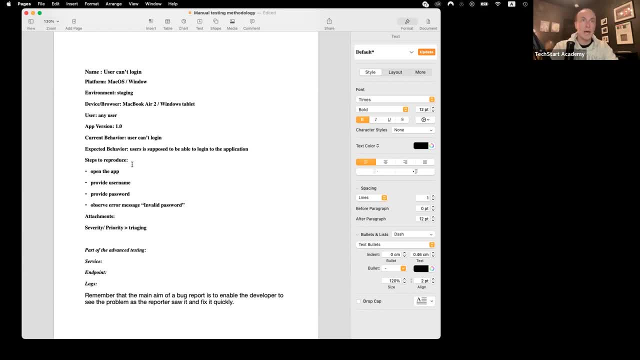 copy your error message: invalid password attachments. you can make a screenshot of this message, like you shared in the chat. so for understanding, here's come trashing. so in this case, like i am a senior qa, for example, like hey, this is the tier zero, uh, it's a uh release, tier zero release blocker. we can't release it. so 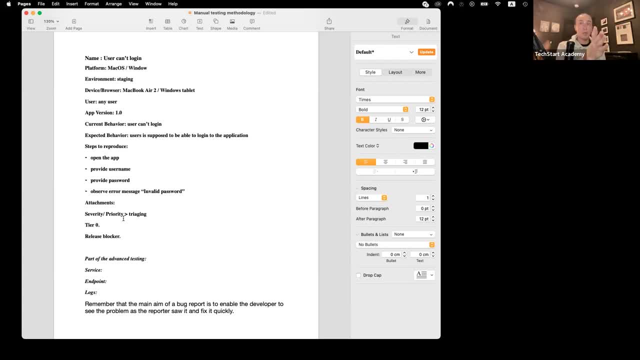 it's gonna look the same everywhere. so here i'm doing like in just a piece of paper, but you will be working and we will work here together on different applications. it's called tracking systems, like jira or, but it's the same. it's the same approach. it's like driving a car: no matter what car you're driving, but it's going to be the 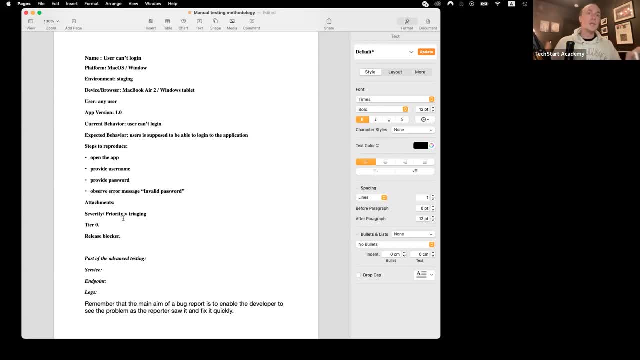 same right, pretty much the same uh. so here, uh, we will discuss it in the part, uh, in our lectures on advanced testing. um, there might be several extra items like service endpoint and logs. we will talk about that later, okay, because it's kind of big deal and you need to know, uh, how to get logs, how to get some calls, what is the service? 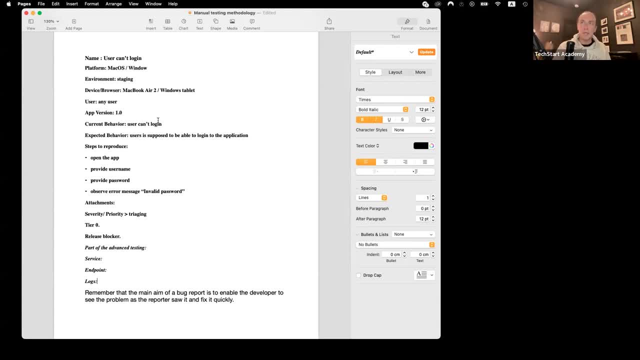 and so on. but here is: it takes like a minute or two just to report. i mean, this bug is very easy. of course it's like talking about um login functionality. of course, sometimes bug reports might be like really long because you need to explain like in details, and usually i do like a 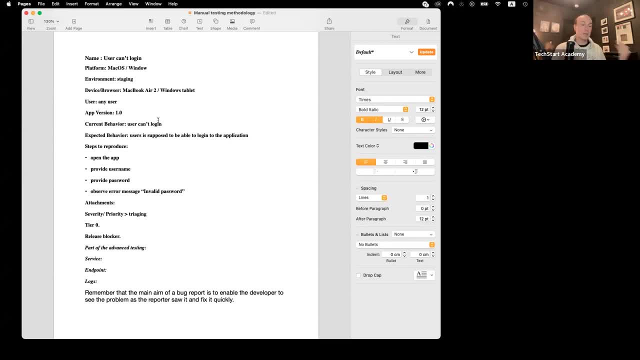 little bit more detail of the screen by providing all the necessary information, because sometimes it's just so hard to follow what is written. it's better just to show it. it's just one more uh, great interview question. you reported a bug, but your developer says i can't reproduce it. it's like 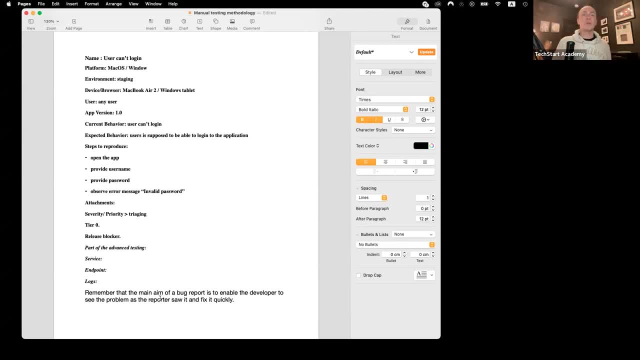 remember that the main aim of the bug report is to enable the developer to see the problem problem and fix it as soon as possible. i i don't know if you've seen the bug report. i don't like these questions. no, i i think nobody likes them, but you need to be ready. 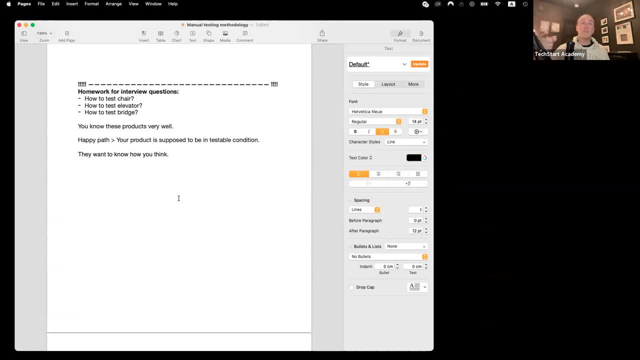 to answer how to test chair, how to test elevator, how to test bridge and pencil or whatever, because i was asked this question several times. it's just crazy. but they people who interview you, they want to see how you think. it's not about like right or wrong, like how chair can be related for testing. but hey, somebody in ikea testing chairs, right. 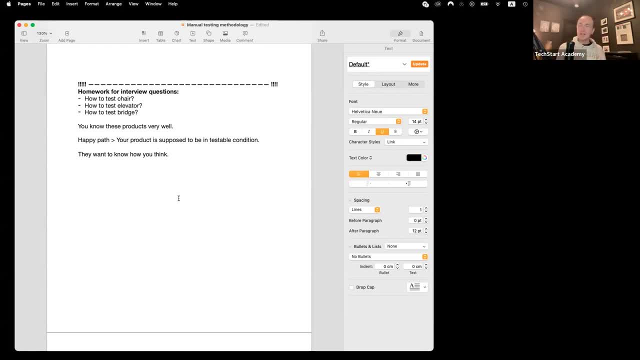 they need to be sure that this chair is made in accordance with documentation, in accordance with uh, user expectations, user experience. um, that's just think about it first. don't try to google it, because you can easily find information, how to test all the stuff, but first just think about it. 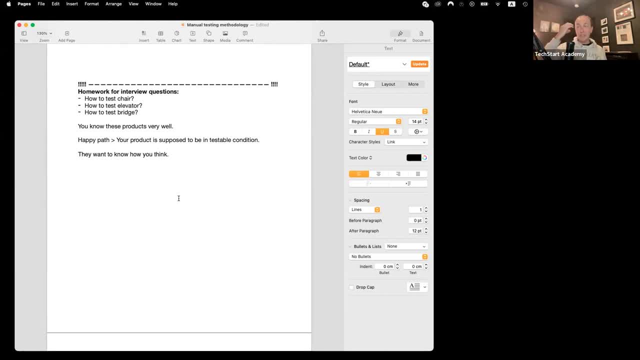 it will give you like a certain mindset, how, how to think about chairs or elevators or bridges in a very different way. you, you, i believe you've never thought about it right. but just uh, and here is um first. uh, think, always, keep in mind your happy path like: why, why do we need a chair? the your product? you're supposed to be in a testable. 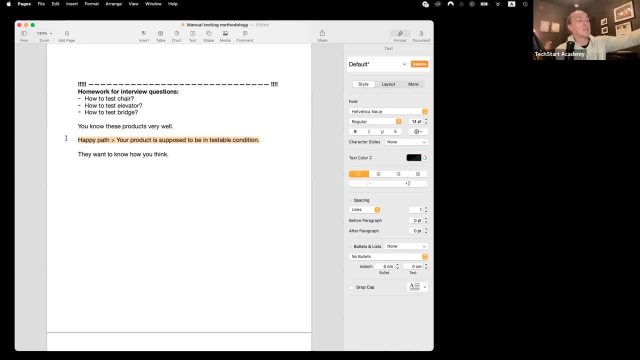 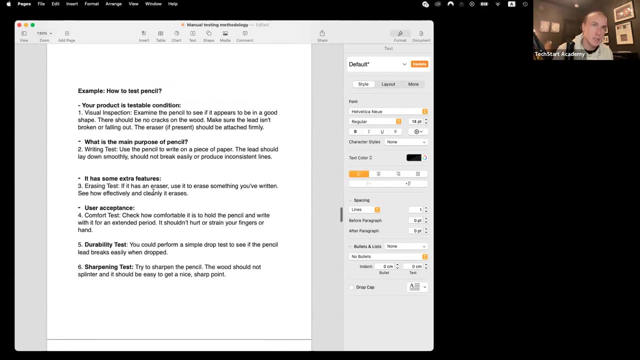 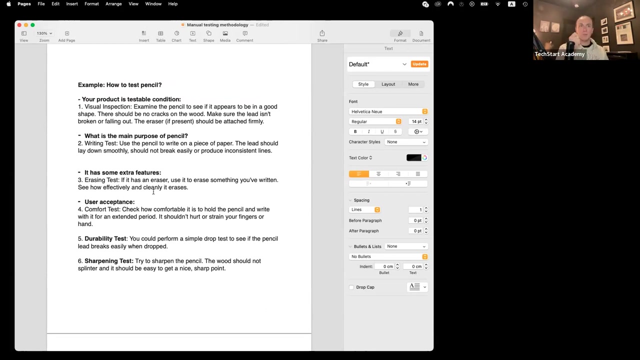 condition, of course. so it means that if we're testing elevator, it's supposed to be electricity in the building. if we're testing chair, it's supposed to be assembled chair, and i'm giving you an example here how to test pencil. just the basic things. so yes, your product is in testable condition, just visual. where is the pencil? I? 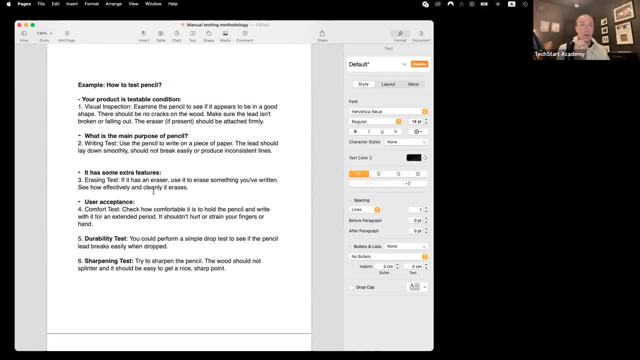 don't have. I have a pen like, uh, this is the pen, so it appears to be like in a good shape, right, so no cracks, it's not broken. like okay, now I can test it. so what is the main purpose of pen or pencil? right, you're taking piece of paper and just start to write, so this is your happy path. 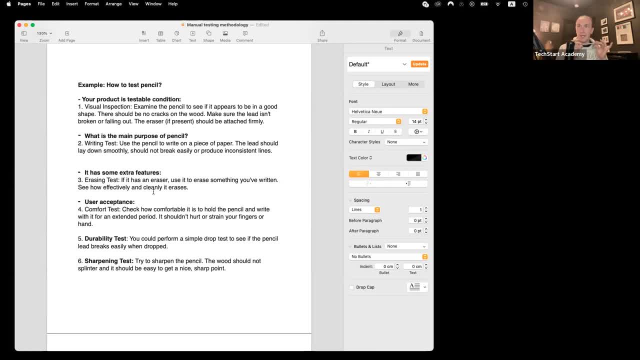 if, uh, your uh object of testing can do the main happy path, you're just like: hey guys, it's broken. thank you, let's test bridge, uh, or whatever. so, talking again about um pencil, if it has some extra features like eraser, so you write something down, then try to erase, because it's it's, it's a part of the. 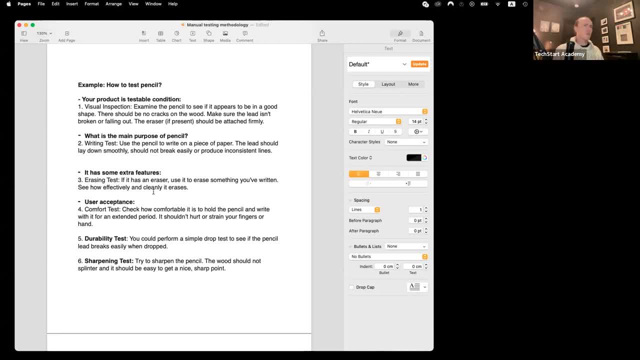 pencil. if it's there, it should work, because I do remember from my childhood some pencils had erasers but they didn't erase at all, they just make, made everything messy and that's it. uh, and then you can go for a very, um, specific kind of testing, like user acceptance, like how it's comfortable, my 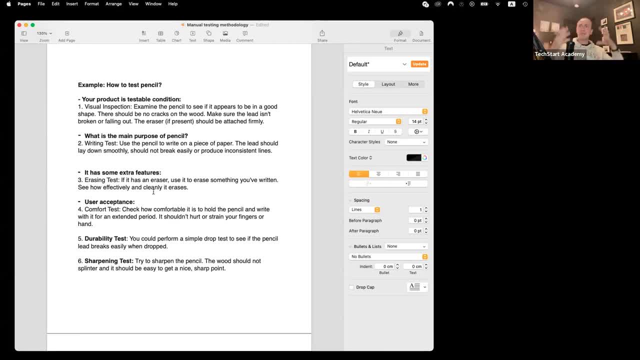 daughter asks me like hey, I wanted this pencil like you be crazy pencil. it's impossible to hold it and write. just this pencil is just about having fun, it's not about write something. so if we are written in our documentation, this pencil is supposed to be fun. kids wanted to want to buy. 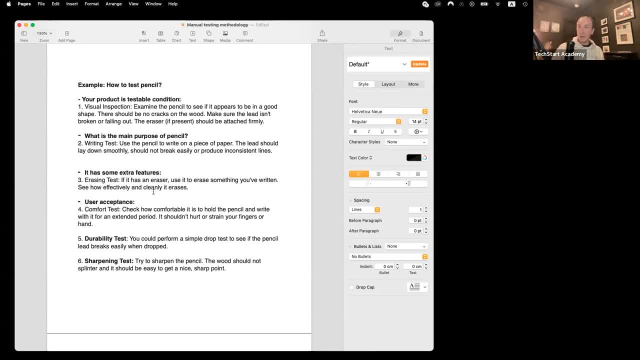 it and play with it, not write with it. yes, it's, it's in accordance with our requirements, but we were talking about just this basic pen or pencil. it's supposed to be comfortable and easy. uh, so yeah, durability test. for example, you can drop your pencil or pen on the floor and if it breaks, like 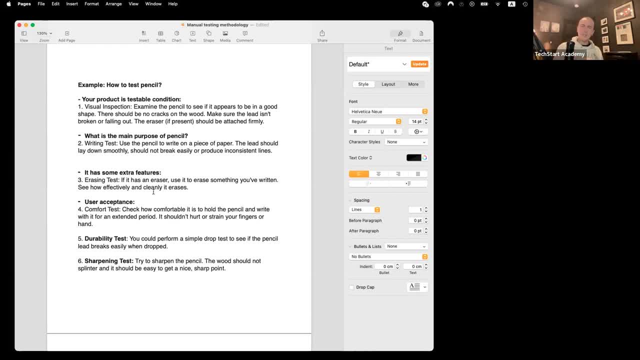 in tiny pieces like: hey, I, I have seen many pencils in my life and I don't remember like breaking them. and then pieces like what is it like? made of glass or what? uh, sharpening test, which is important, so I want to sharp my pencil, take by by a sharpener or a knife, so I should be able to do this if I know how to do this. so just, 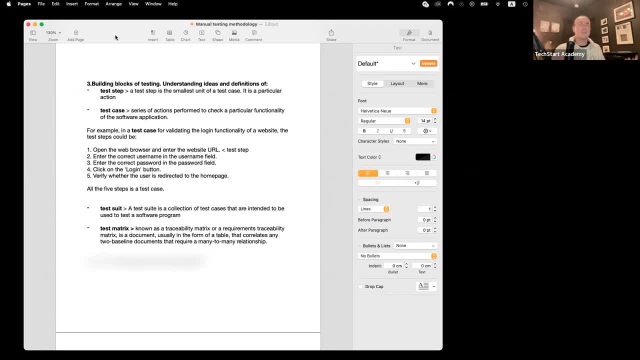 and it's about like how to testing pants, chair, whatever. so just try to think about it and answer these questions, uh to yourself, um, and then you can Google some- I wouldn't say answers, just Google ideas, because some people they're doing crazy things about this testing. they have, like I have like 45 different types.